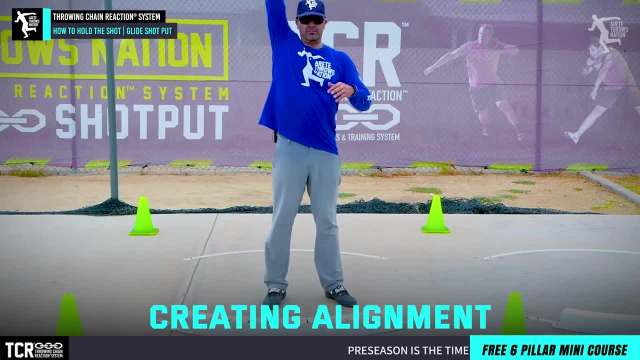 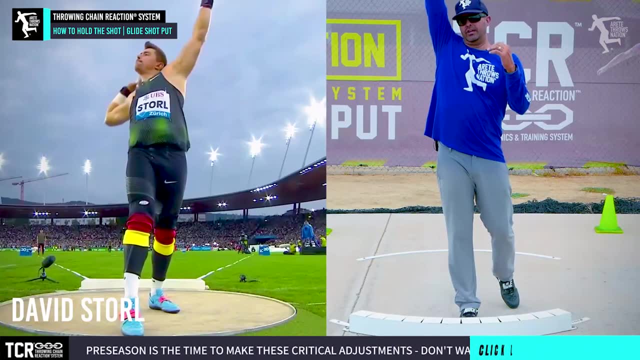 the things we talk about is creating alignment, So we want to practice. you're gonna see most elite shot putters and you're gonna see what we call as they set alignment. So one of our favorite is Valerie Adams. David Storrell looking at: 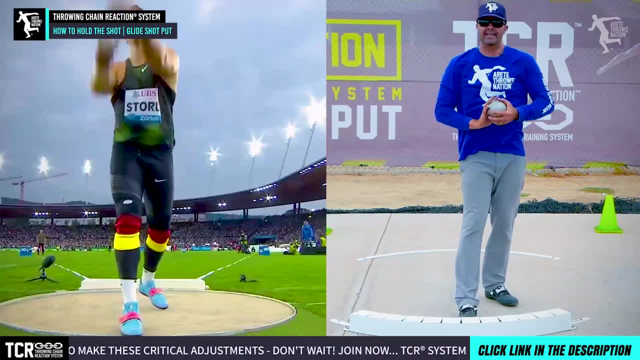 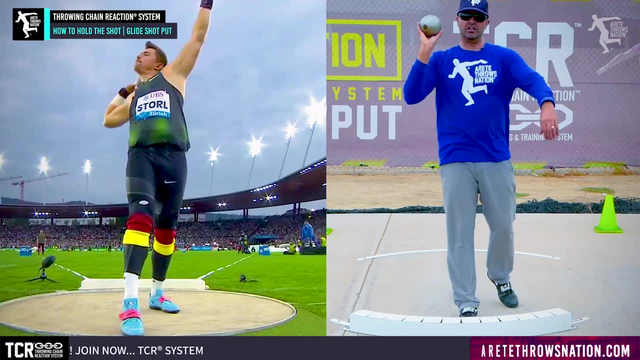 classic gliders like Werner Gunther. So you're gonna see how they get the shot. they get it up here and they create and they find that spot and they're bringing the shot down and you're gonna see this hand position here. 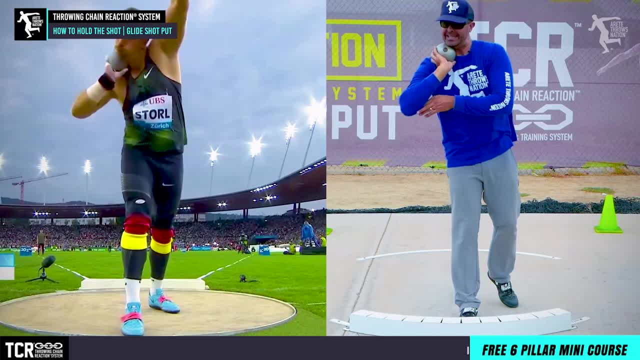 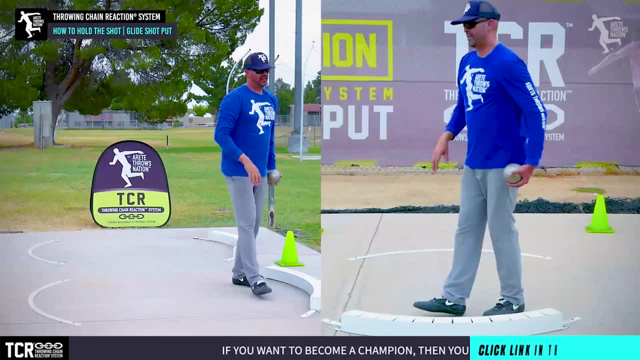 and then what they're gonna do is bring it under. You're gonna see that the elbow is away and again, where's the crease of the elbow? We're in this position. So the deal is why we don't want to see our arm like this or like this Sometimes you 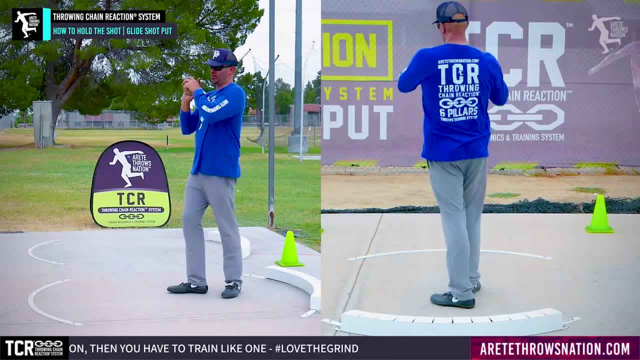 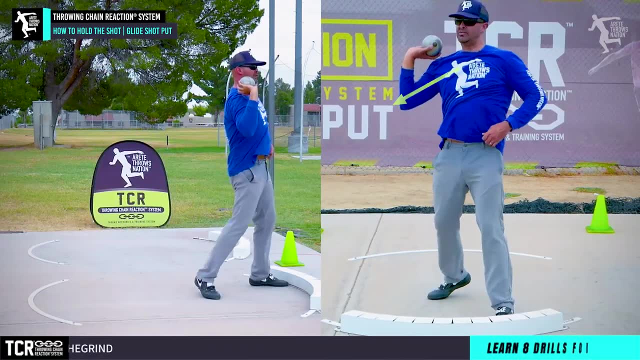 see kids doing this, or you'll see gliders- right, We'll see your gliders holding the shot like this. so you're gonna notice, when I try to come out of this position and I'm here and my elbow's here, that's gonna cause the shot to come out. Okay, so one of the things you want. 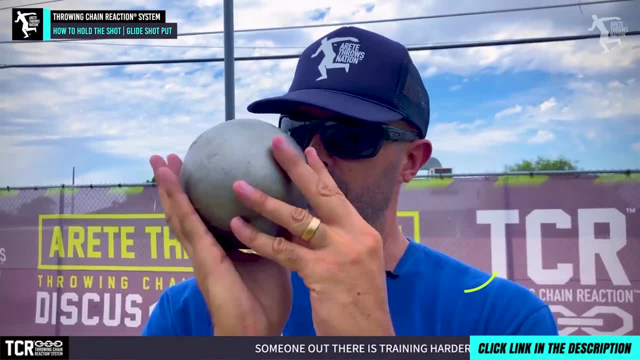 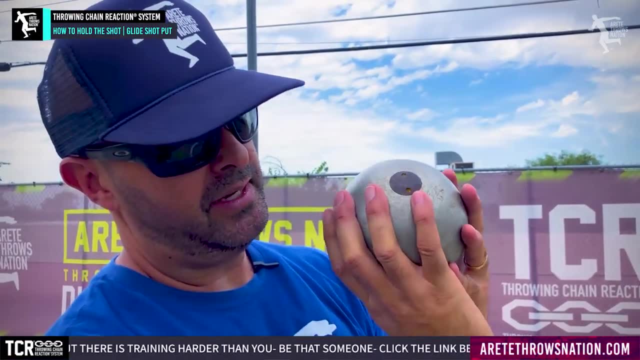 to be focused on again is you're gonna see how we've got this shot sitting in here and how we have the fingers sitting like this. Now you're gonna notice that the ball is gonna be sitting here. Sometimes the pinky. the pinky is sitting. 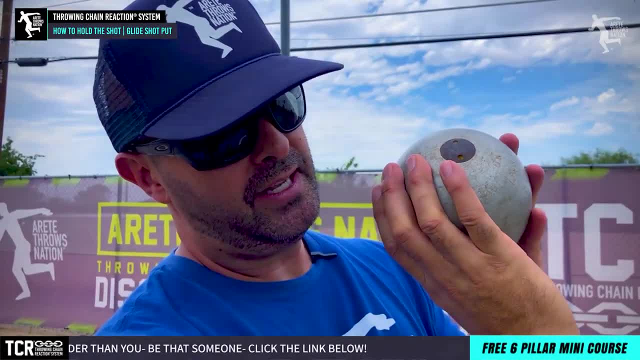 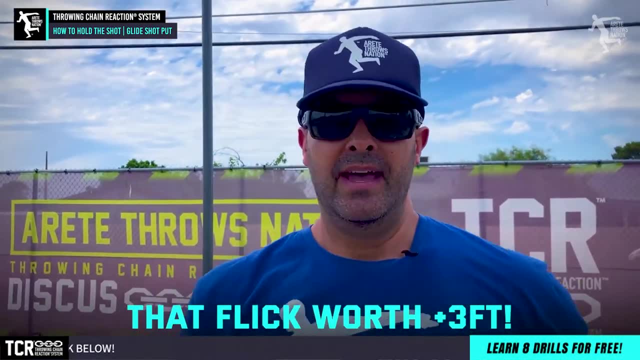 a little bit to help some stabilization. but you're more elite guys. they're gonna get that finger closer so that they can get more of this type of thing, and so you're gonna be able to put more force. That flick is worth an extra. 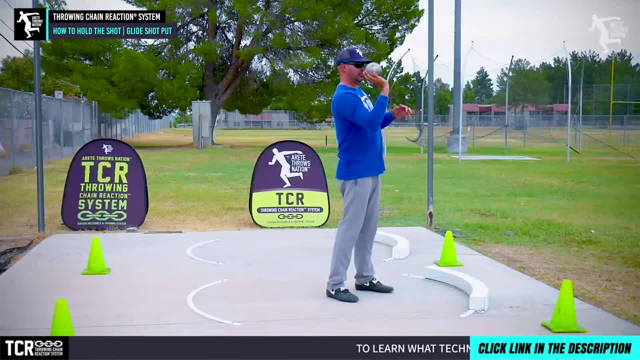 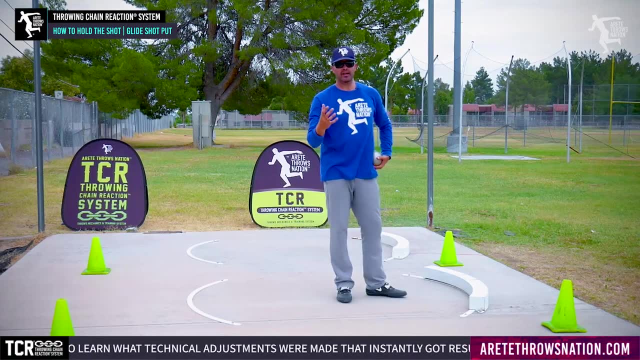 foot to maybe as much as three feet. The second thing we talked about is, once we get that right, we want to be able to understand that where it's gonna go in the neck. This is gonna be somewhat thrower-centric, right. Some guys are gonna 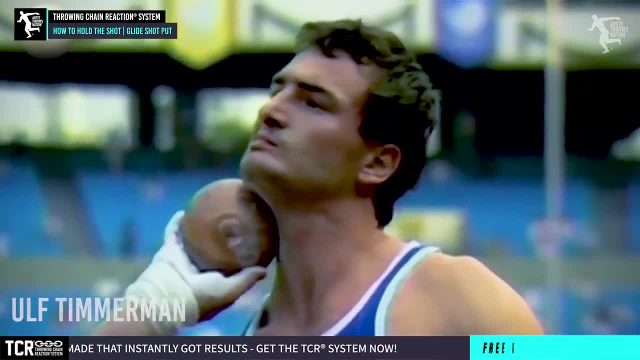 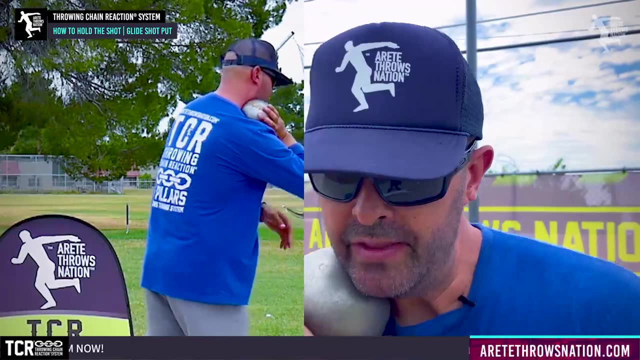 like it a little lower. If you look at the glide legend Ulf Timmerman- he was down here- You're gonna notice where the elbow is, though. So now, what you're gonna notice is when I hit that, and you're seeing where the elbow position is. so if 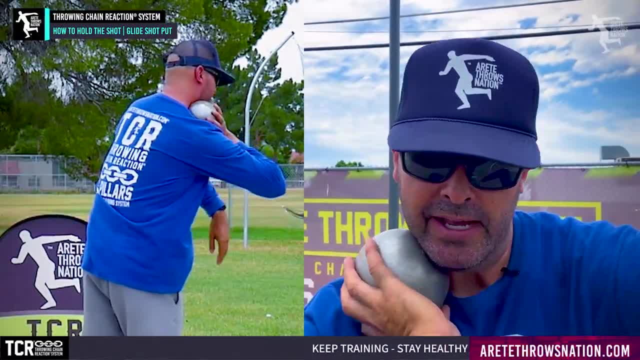 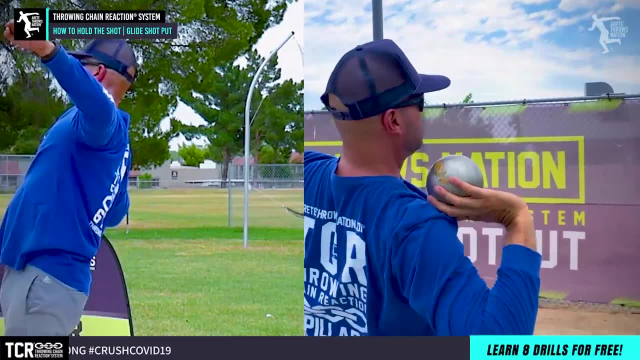 I'm gliding and I bring that shot down and you see me here and you're gonna see that now I'm in this position because as I hit the glide and this opens now I'm gonna be in this position to pull in that nice linear strike position. So 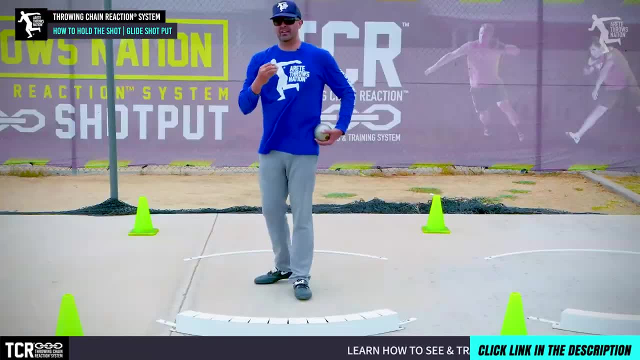 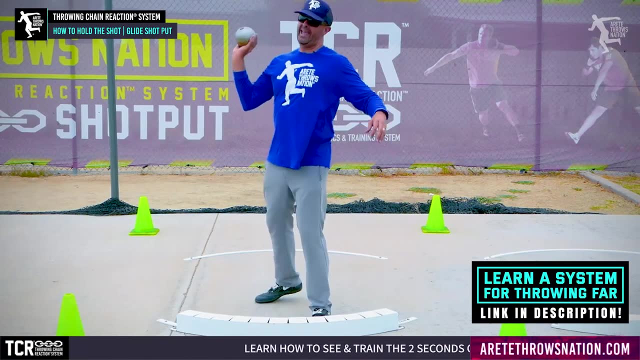 basically what we wanted to help you guys understand is that there's a lot of little nuanced details to holding the shot. It really is the first thing, and what do kids want to do? They want to get in right away. and why does that shot? 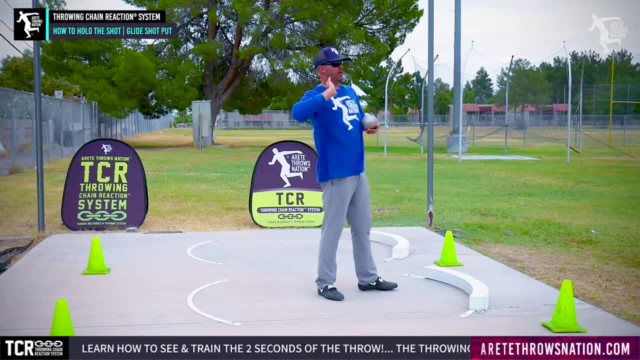 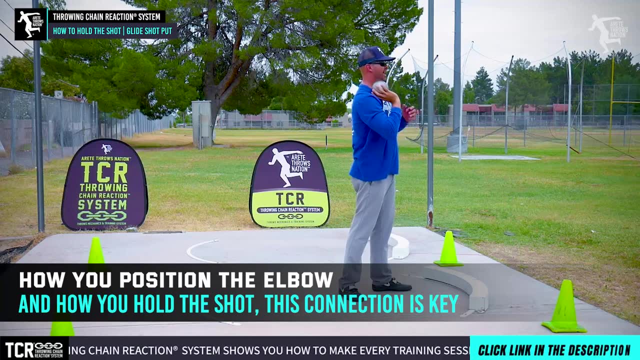 come out, Because if you learn the rules of the shot put, the elbow has to be up, it can't come off the neck, you can't throw it. Well, that's gonna be because of how you position the shot, The elbow, and how you're holding in your hand, and this connection is what's gonna 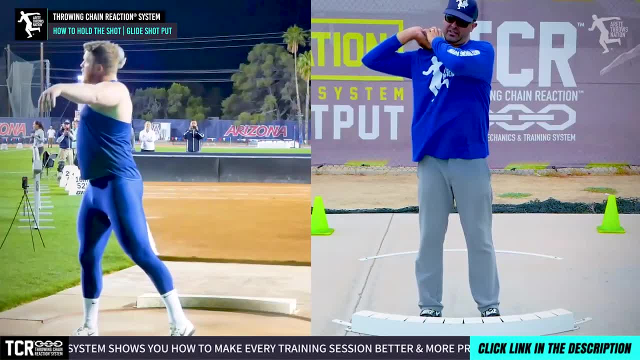 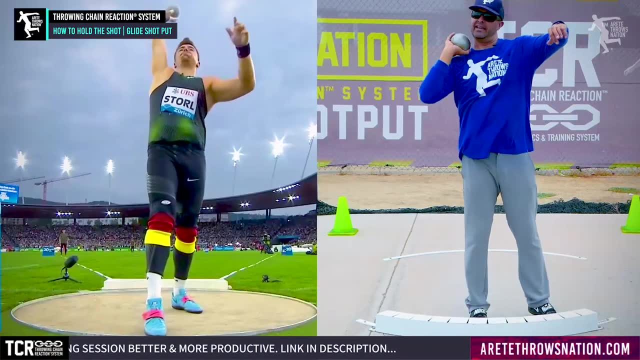 be key. So this is why you'll see your rotational throwers, the big muscular guys. they're gonna see, you're gonna see this and you're gonna see that that arm is level and in the glide. you're gonna see this kind of thing and you're gonna. 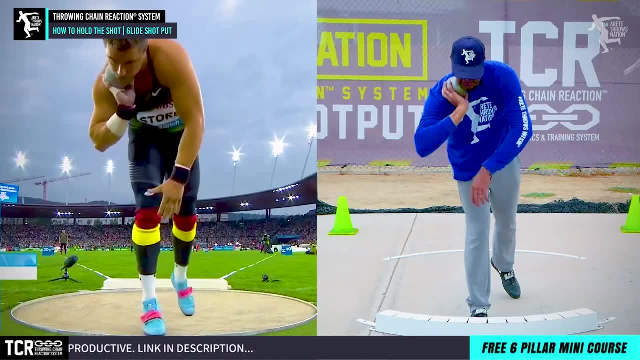 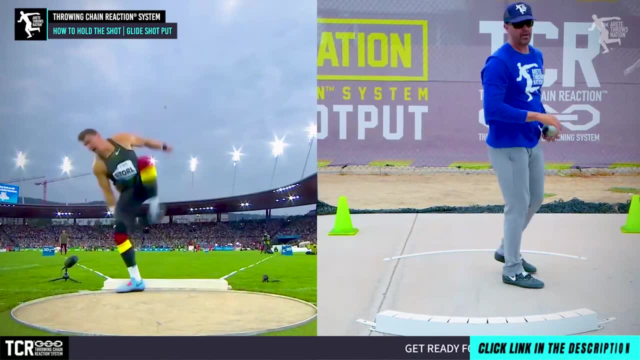 see that elbow kind of here and they're carrying it more in this position. So when they line up and they're gonna move into the strike, you're gonna be able to get behind this point and push the shot through. How you hold and how you grip. 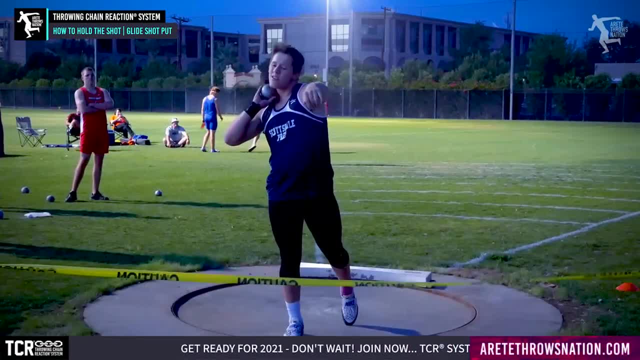 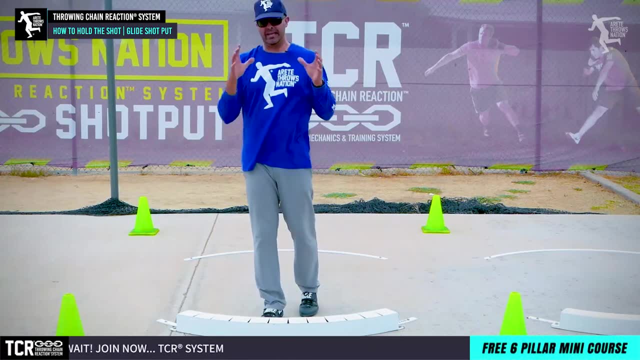 have a huge impact. If you don't get these two things right- how the hand position is gonna work and how the angle of the arm and where the arm is gonna sit- it's gonna completely make learning technique next to impossible, because 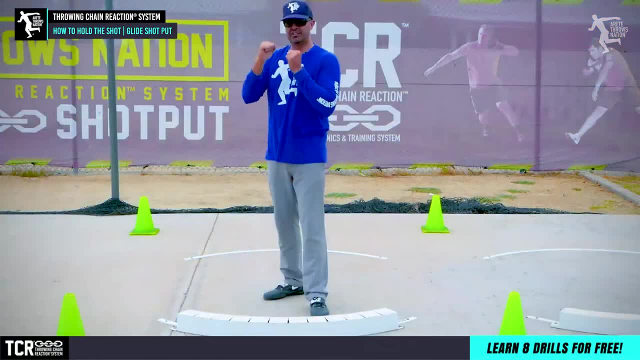 you're always gonna be feeling the weight of the shot pulling away. it's always gonna change how you move, it's gonna change your balance, it's never gonna allow you to strike the shot clean. and if you're doing that, then you're. 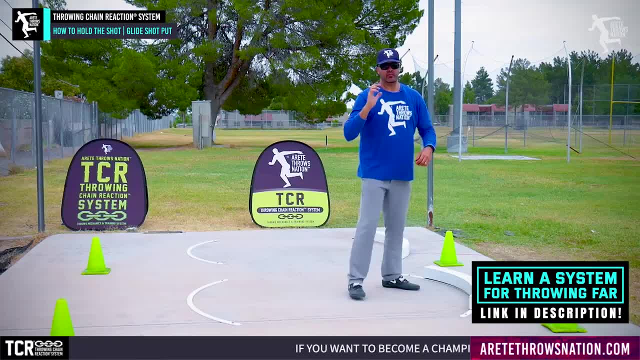 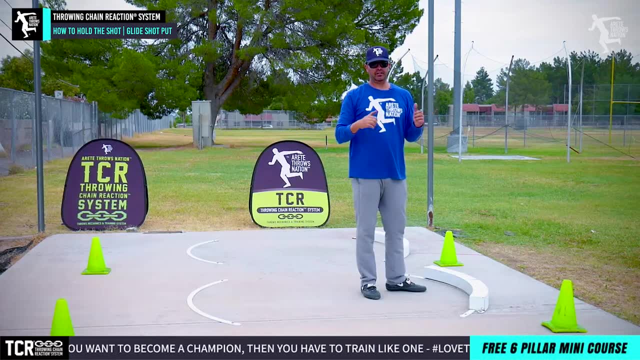 always gonna compensate, right, Because if your arms out of position, then what you're gonna wind up doing? if your arm drops, well, then you're gonna be trying to get yourself into a putting motion, which is clearly not going to help you. 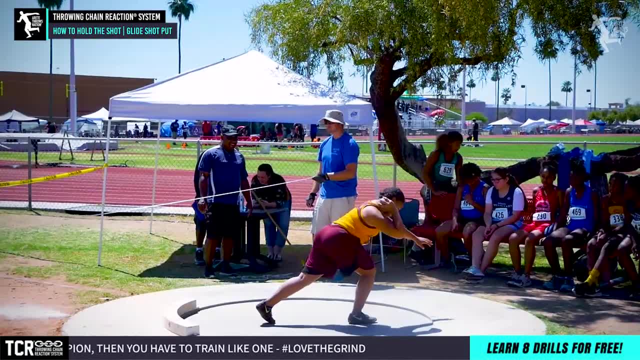 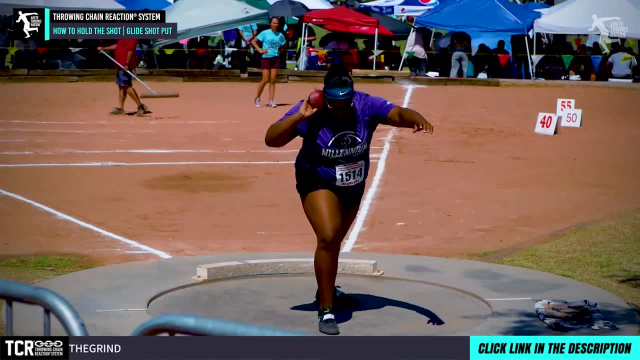 develop a good technical pattern. So again, this is something we talked about in the throwing chain reaction. it's a real simple thing. we teach a four-part sequence how we're gonna get everything set up, and so we get everything in position, and we've seen a lot of that. So the elbow stays. 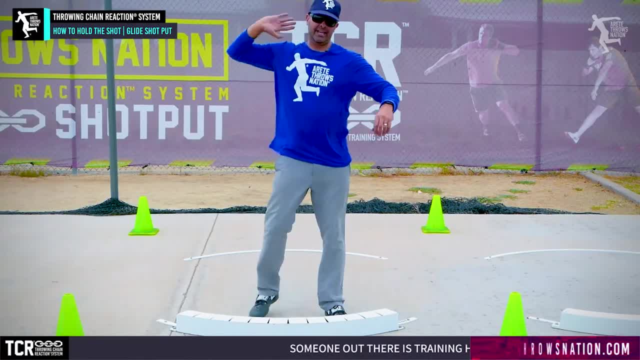 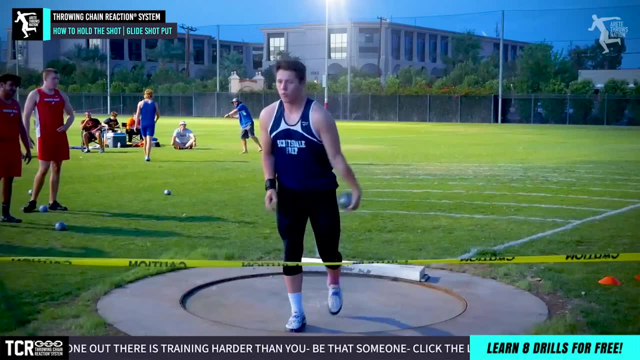 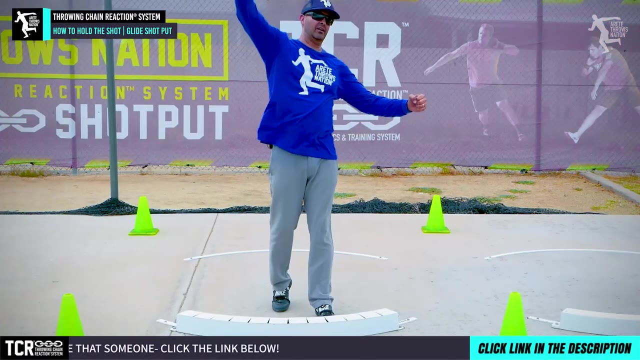 down and away and in the rotation. it's up here because we have two different angles of release. We're really looking at about 36 to 40 degrees in the rotational shot and we're really looking at two degrees is in that range in the glide we want to be a much. it's a higher angle of release. so 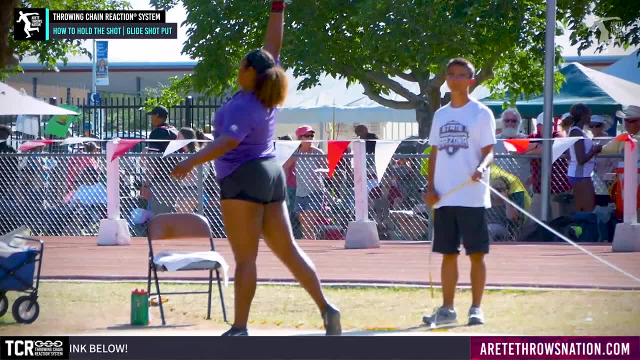 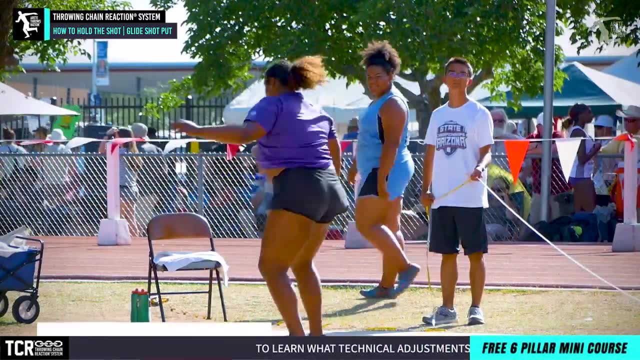 you're going to be seeing, because it's a linear delivery and out and the rotation is about speed and a longer path to generate speed and power. so those are the two things, but you've got to get this hand position right. you've got to get this elbow position right, because if you don't, it's